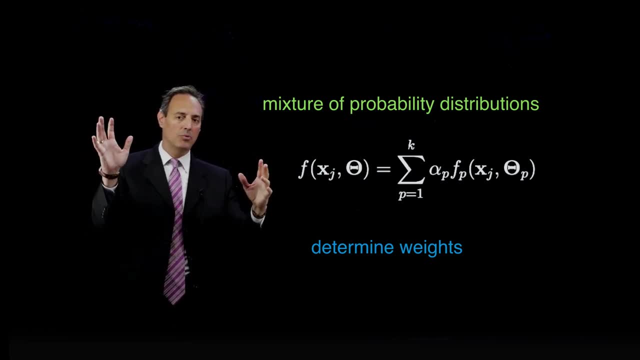 are there. Remember, just like as in k-means, k-means required to make a choice about how many clusters there are. Hierarchical clustering also required you to give some kind of threshold or some kind of information about how many clusters you might want. This also is saying how many probability distributions. 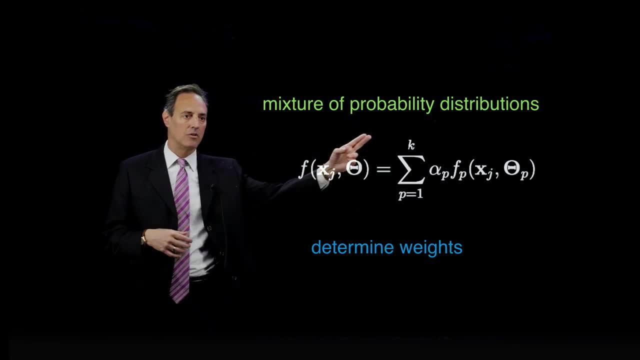 do you think you need for that data? So that's determining k. and then what is the form of the distribution? So you're going to impose structure in the form of the model. Normally, a lot of times, what we do is we make f of p be, in fact, a. 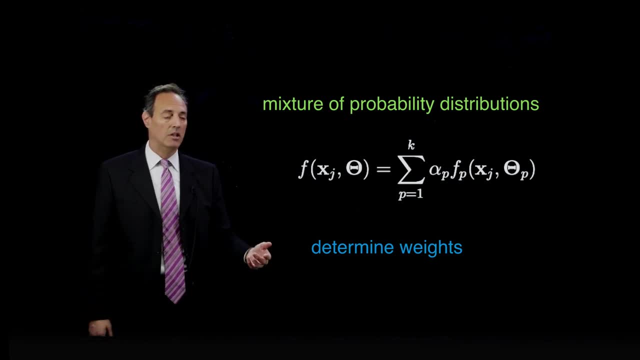 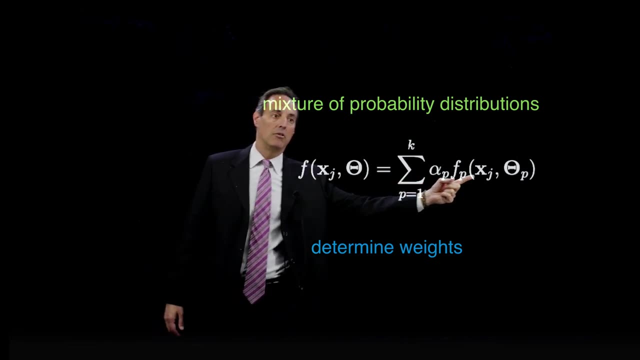 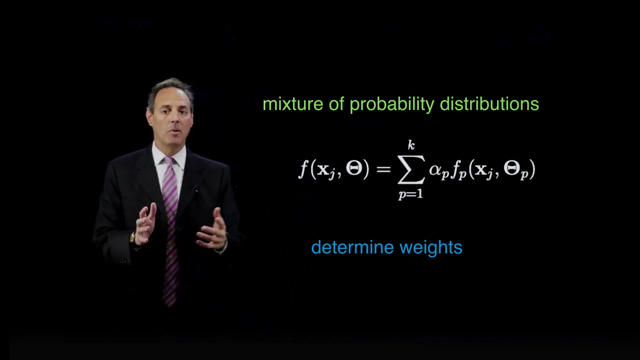 Gaussian distributed variable, And so what we would need to do, then, is simply determine what are the weights between the distributions, determine those alpha p and determine the parameters of each of the distributions, And, of course, we're going to do this through optimization. Remember, this is a 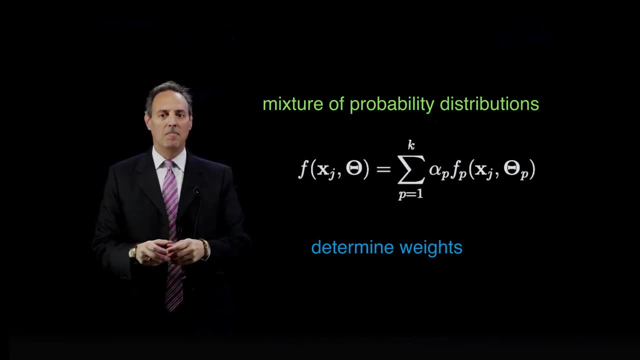 regression problem, just like we talked about in chapter 4.. I have input data, I have the distribution, and then I have the distribution And then I have the output data. This is the model, right there, My model is a sum of distributions. 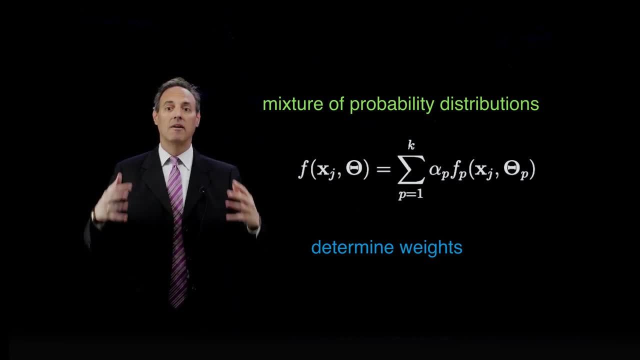 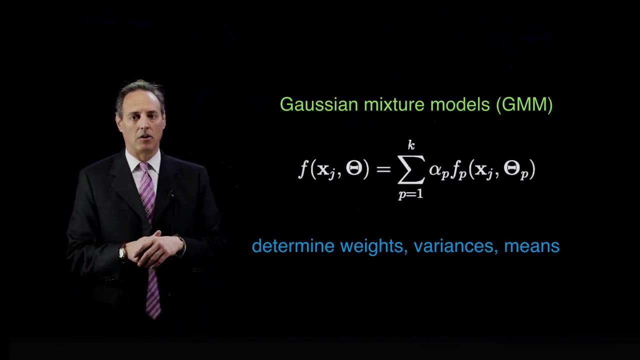 where I don't know the parameters of the distribution or their weights, Find those. That's the optimization problem, such that you best match the input to the output of the data. Okay, Now what oftentimes happens is you assume that these f of p's in fact are Gaussians. Okay, Normally distributed variables. so 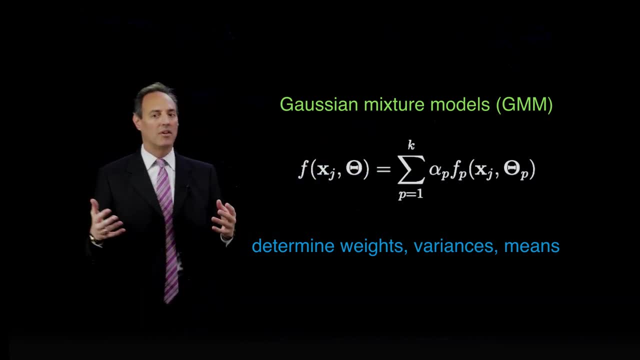 in fact, Gaussian mixture models, GMS and so on. So what you're going to do is you're going to assume that these GMS are kind of one of the important classes. If you have nothing better to guess about your distribution, you typically assume it's. 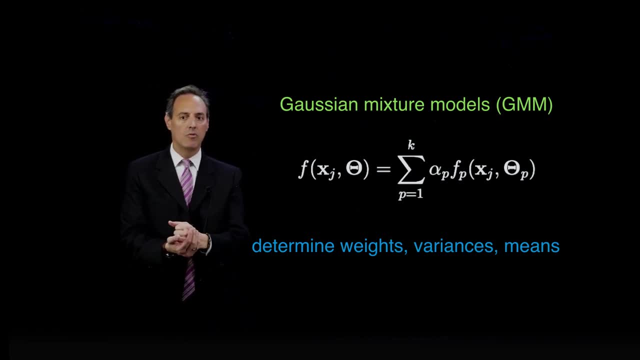 going to be normally distributed right, Characterized by one, two numbers, a mean and a variance. There's no reason why you pick some kind of more complex or harder probability distribution unless you had information to why that choice should be made. So generically, what people do if you know nothing else, pick a normal. 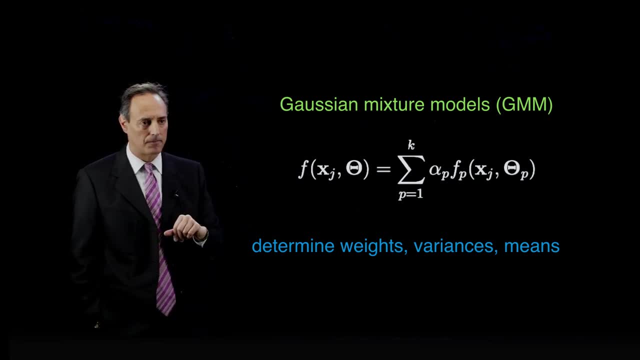 distribution, which has a parametric distribution, And then you're going to use that parameterization by two parameters, a mean and a variance, which are things you can very easily compute for distributions as well. So your goal, given that, determine the weights, the variances, the means. So, if I assume that, 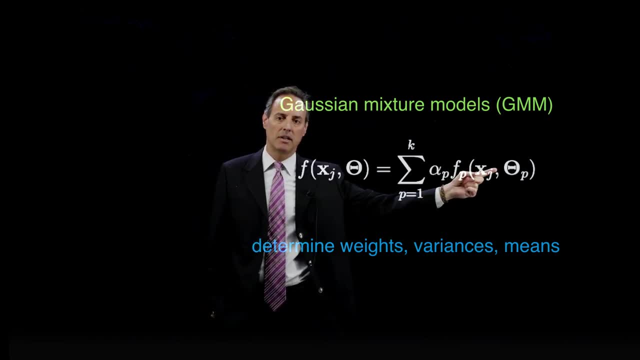 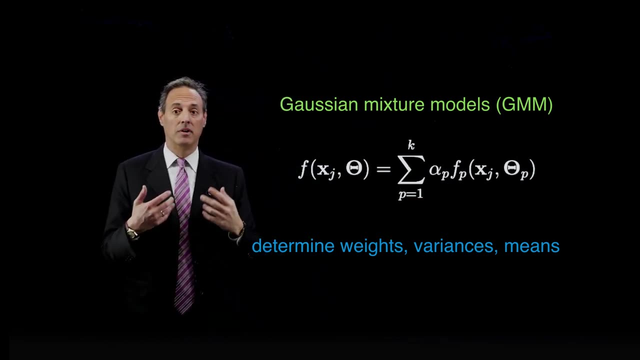 this is a Gaussian distribution or normal distribution, then I have a mean and a variance for each one plus a weight, So three parameters I have to determine. So if I have a mixture of two Gaussians, then I have six total parameters I have. 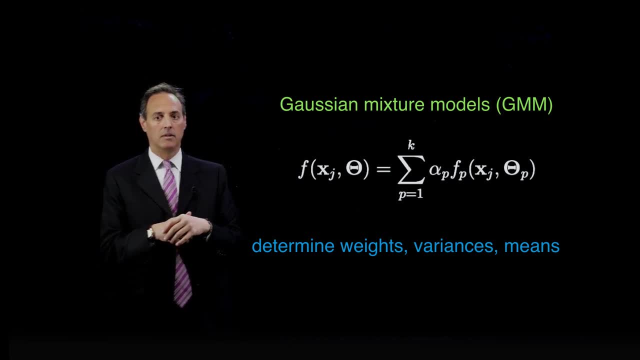 to determine In order to get the best fit to the data. Okay, hopefully that makes sense. So the nice thing too about assuming that is it's a fairly well constrained optimization problem: There's a fixed number of parameters you have to determine through the optimization. 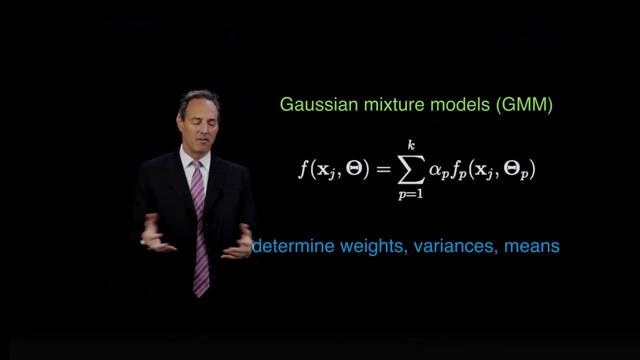 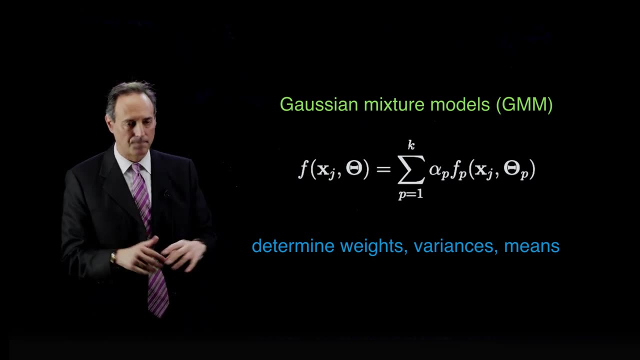 procedure and in almost a minimal set of parameters, because one of the things that's nice about normal distributions is: two parameters are all you need to characterize the whole thing. Okay, so we're actually going to do Gaussian mixtures here for some data, So we're going 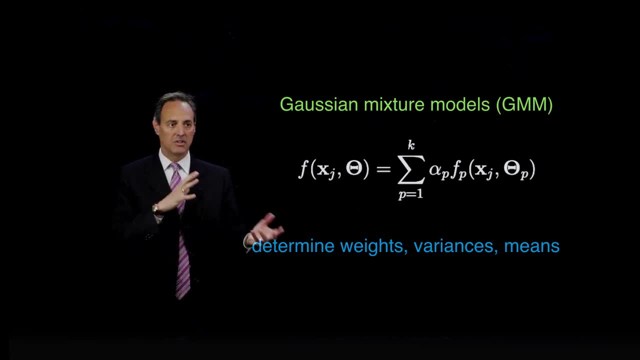 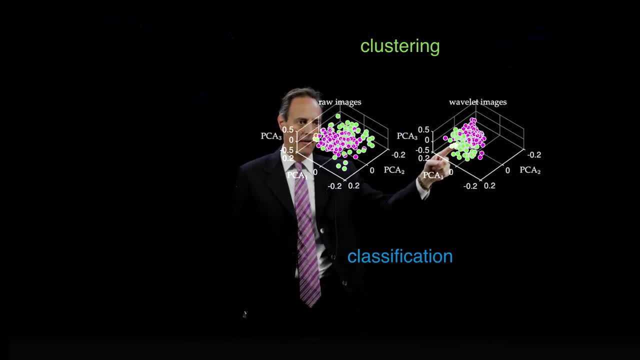 mixtures here for some data. Okay, so we're actually going to do Gaussian mixtures here for some data. Okay, so we're actually going to do Gaussian mixtures here for some data is if I want to do some clustering here. 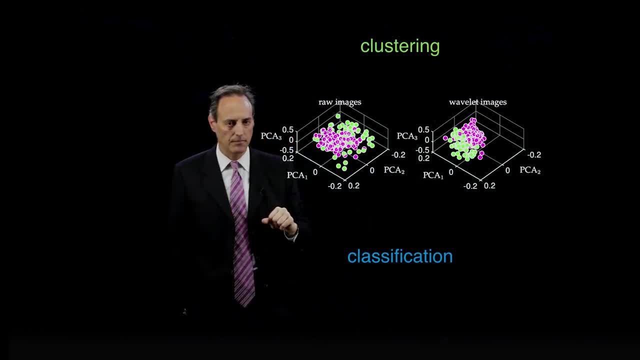 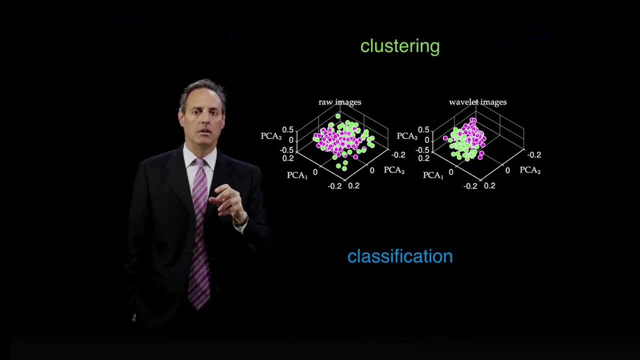 you might say there's a Gaussian here and there's a Gaussian there, Or normal distribution in each, and you could say: okay, I will make two clusters and I will find the best two normal distributions that, if I add them together, produce the data that I see here. okay, 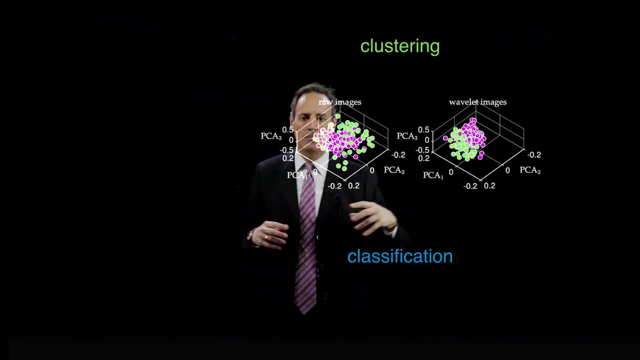 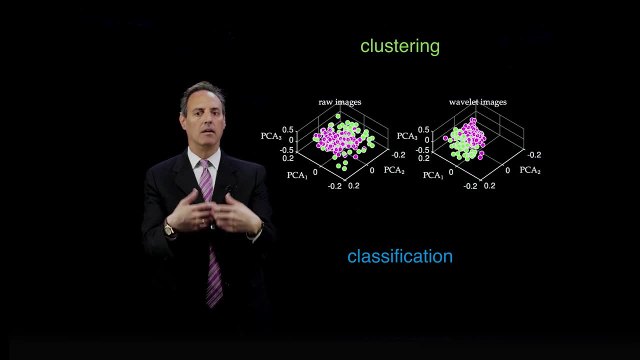 So right away you can start seeing that the structure you see in your data is actually what's motivating you imposing that there is in fact a probability distribution describing that data. okay, Notice that this is very different than k-means and hierarchical clustering. 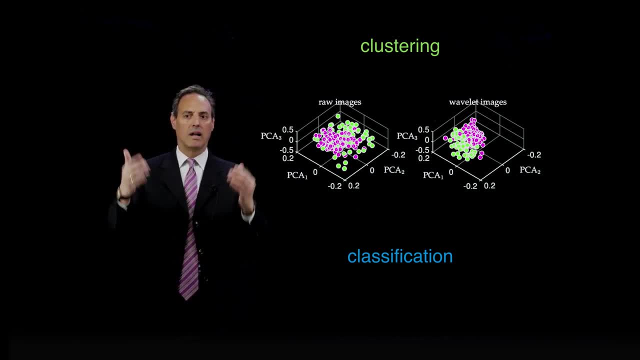 In those. there really was no optimization, It was just simply executed algorithm. straightforward Here, this E&M algorithm is trying to find you a probability distribution, or approximate a probability distribution, There in k-means and hierarchical. it just simply cut it through. 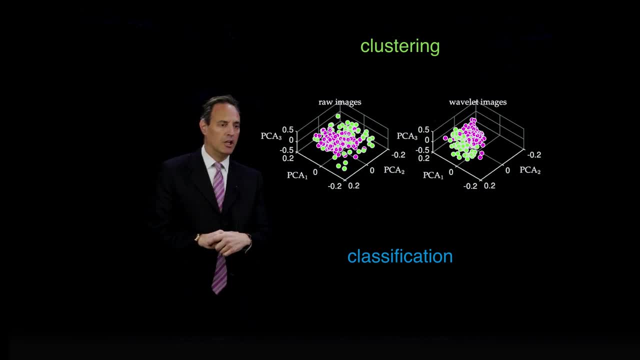 tell me where the data belongs. Okay, so the idea here is: once you have that, you can start thinking about. I now can build classifiers out of that data in an unsupervised way because I have the probability distributions of the various components. that's making up the data I see. okay. 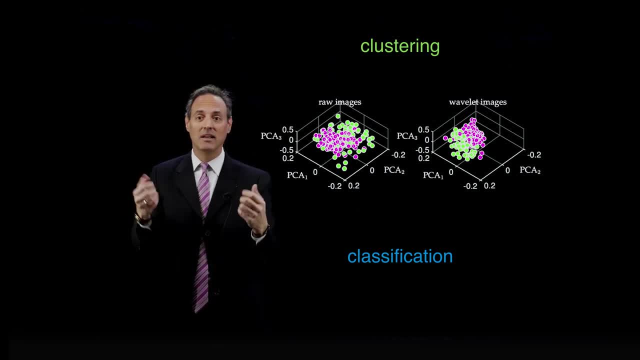 And it's an assumption. So if you have two clusters, the idea would be there's probably two probability distributions describing those clusters that if I add them together it will be a probability distribution. So if I add them together it will be a probability distribution. 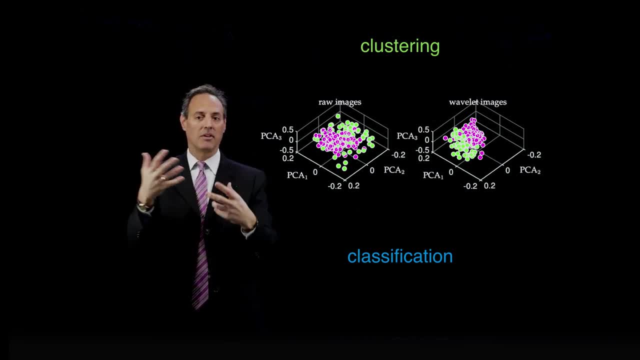 So if I add them together it will describe the overall data set. If there's three clusters, you might think about three probability distributions. that would describe that data set. You have to pick the number of probability distributions to put in, So just like k-means. 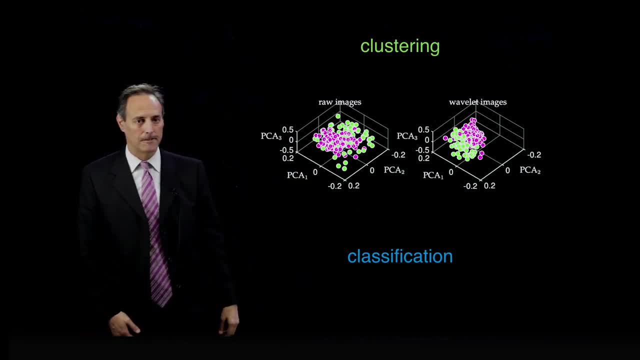 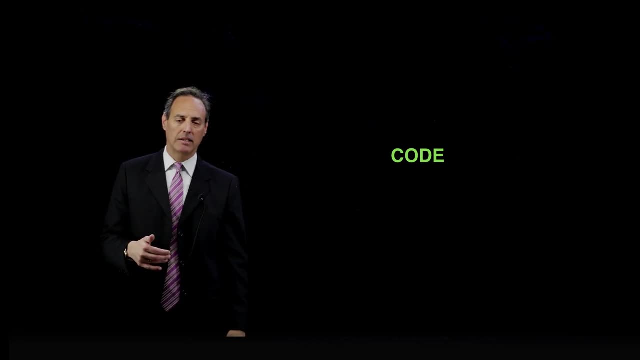 you've got to pick the number of clusters. Here you have to pick the number of probability distributions. All right, so let's go through some code. I'm going to show you how this actually looks in practice. We'll run through a Gaussian mixture model code. 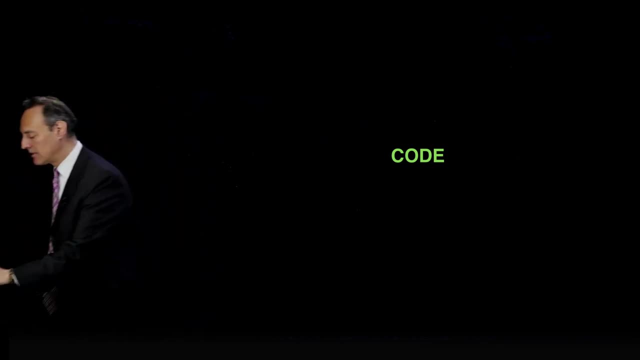 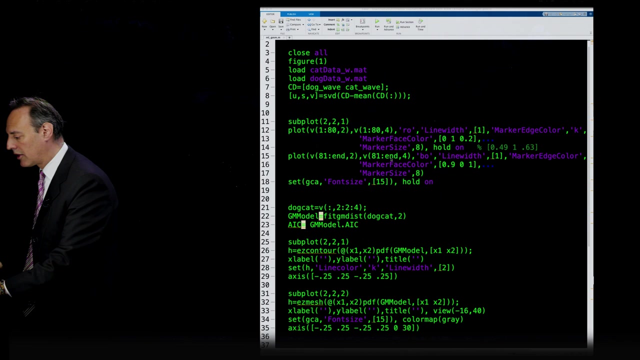 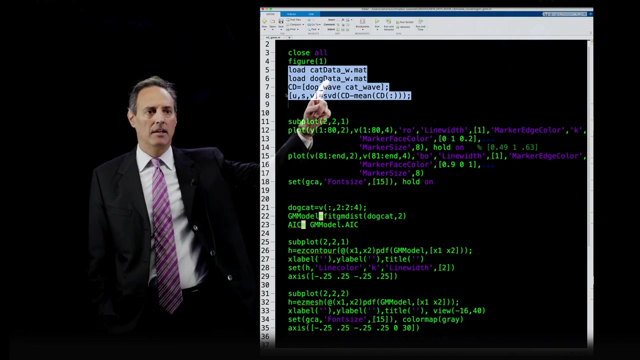 It's very simple. It's very simple to implement in MATLAB or Scikit-learn or any of these Very powerful. Okay, We are going to start back at the cat and dog data. So first of all, here it is: Load cat data in the wavelet domain. 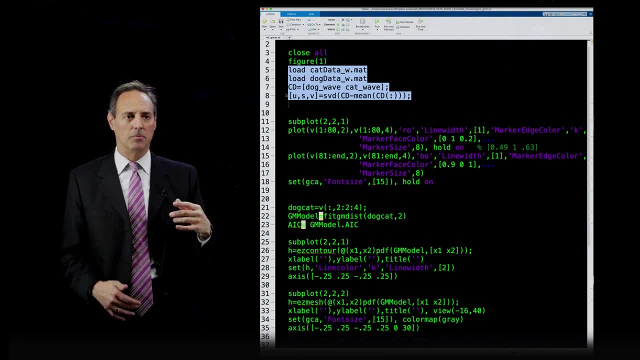 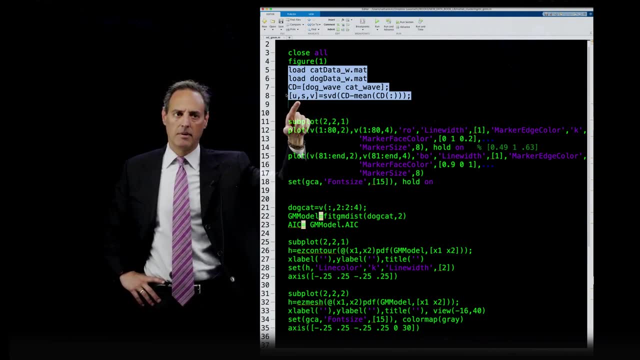 dog data in the wavelet domain. Remember that in the wavelet domain it was much more distinguishable about whether you have a cat and dog. So I'm going to take the dog data, cat data, concatenate them and project it into a low-rank subspace by doing the SVD. 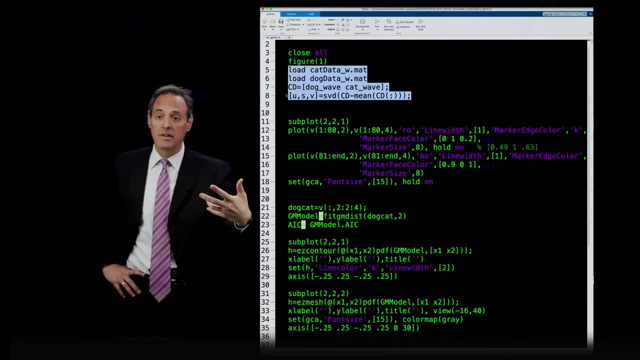 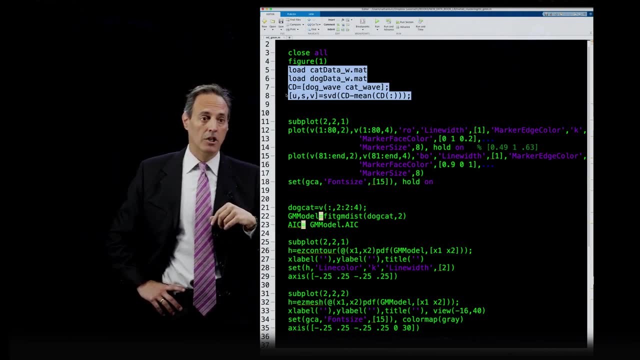 Okay, So I take the data, I do the projection. We've already done this in the first lecture of this chapter, section 5.1.. So I'm just playing out from there again So I can plot all that. and this is what this is doing here. 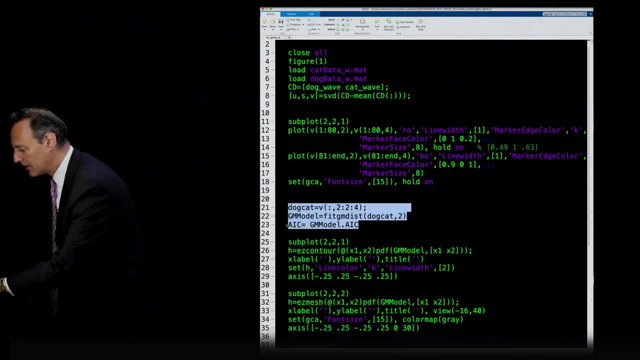 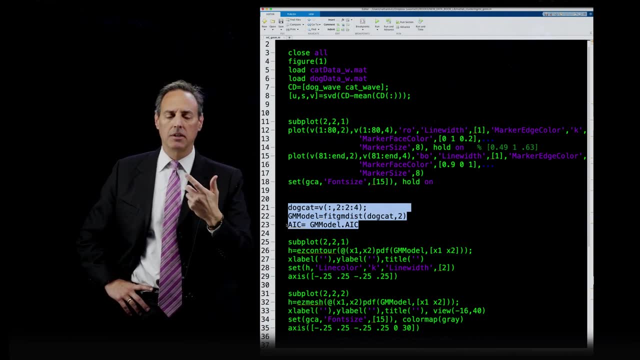 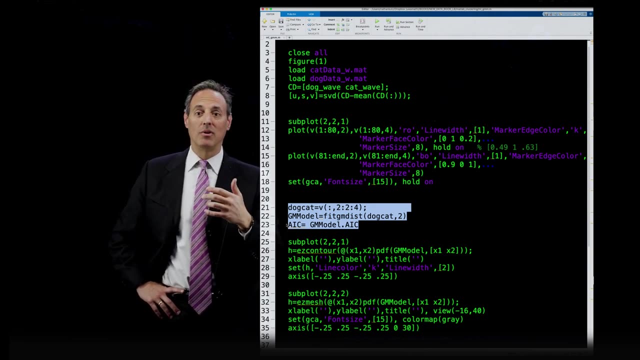 Now what I want to do is say: okay, let's come to here In particular. one of the things that happened is when we projected- and this was from lecture 5.1,, but I'll highlight it here- When we actually projected onto modes 2 and 4 specifically. 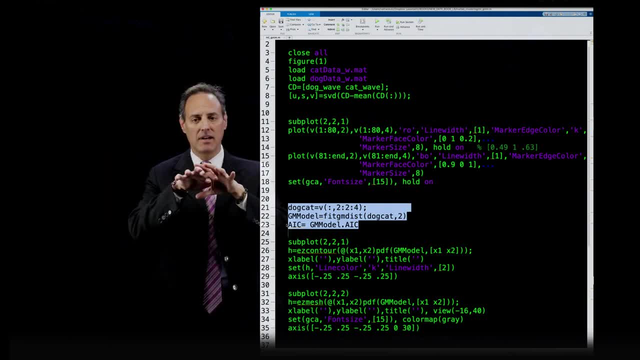 they especially with the wavelet data. those were the two data sets that had very nice separation of the probability distributions. So if you go back and look at that lecture, it's very nicely separated, And so what we're going to do is: 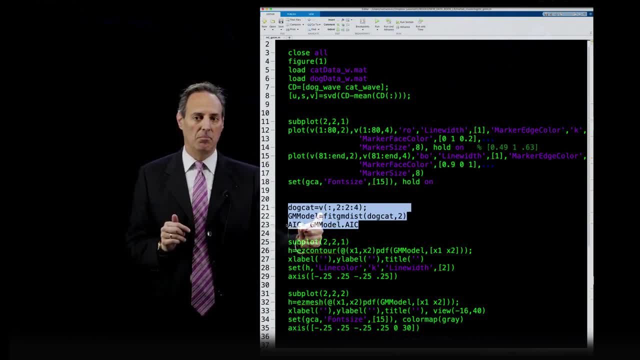 we're going to come over here and take the V matrix from the SVD which tells us about that projection, and we're going to go take, take column 2, skip by 2, by 4.. So this is going to pull out column 2 and 4.. 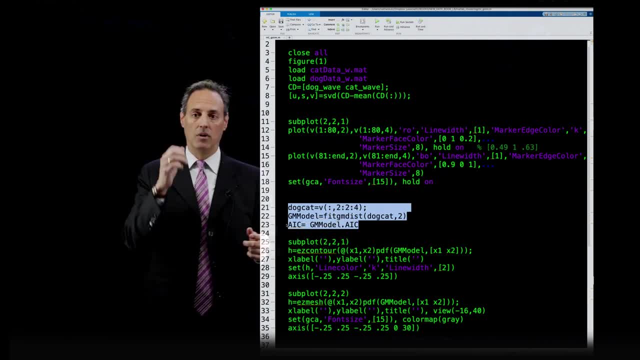 So, okay, right, go to column 2,, skip 2, go to 4.. So go grab those two columns of data. and this is the projection of the cat-dog data into modes 2 and 4 of the feature space. 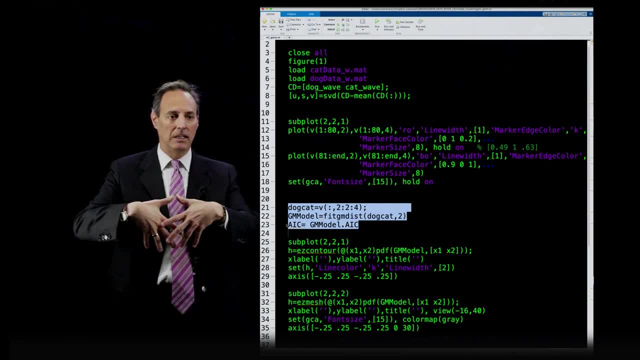 And those are the ones that seem to have the highest separability of the PDF, And what I'm going to do is basically build a Gaussian mixture model based upon those two features of the data. So mode 2 and 4 in the SVD modes. 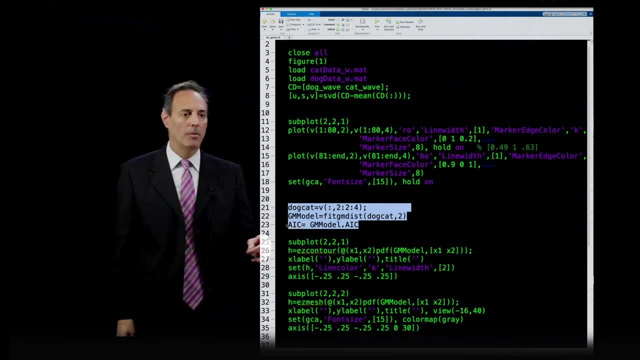 or PCA, components 2 and 4, okay, So here's what we're going to do. This is how easy it is: Fit gm distribution dogcat, which is what the 2, 4 column to probability distributions, And that comes back as gmm model. 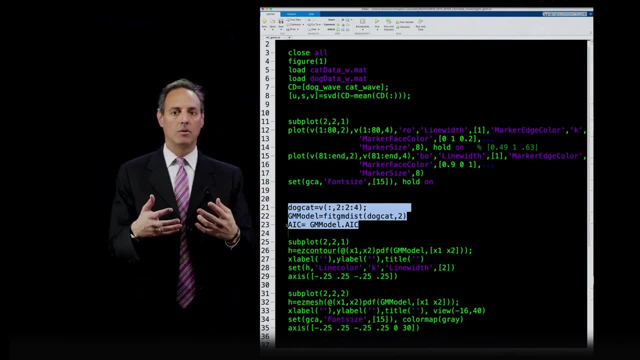 So that's it. So you just want to say- I'm going to fit it to- to probability distributions go And it's a Gaussian mixture model. So gmm means Gaussian mixture model. So I'm already assuming it's normally distributed variables. 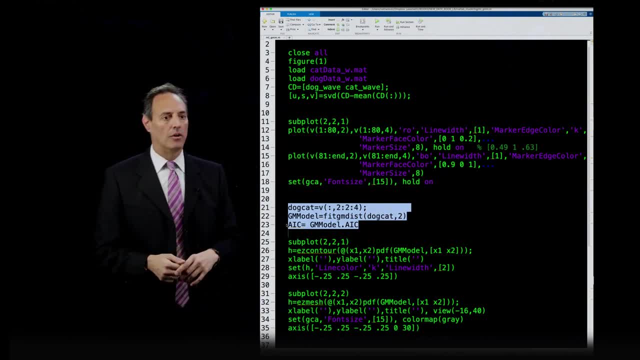 Okay, with essentially two clusters. So if you do this, you're going to get out this model And I'm going to plot the results of the model, But also what's interesting about this gmm model: you can actually get out for yourself the AIC score. 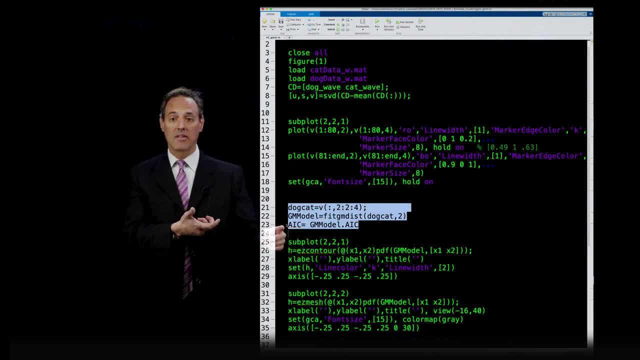 In other words, the ICAEK information criteria will come right out of this, So it can tell you how good that model was. So this is really nice to have this built in as something that computes as it does it. So gmmmodelaic will give you back the AIC score for this fitting procedure. 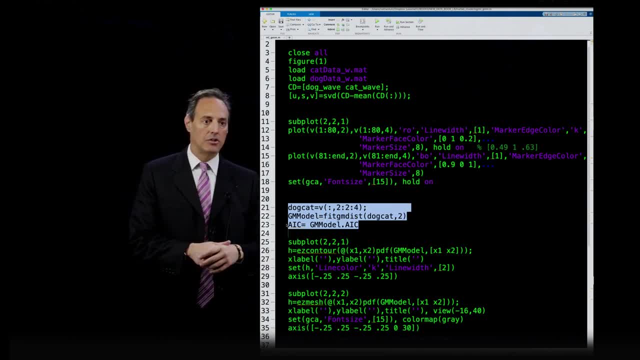 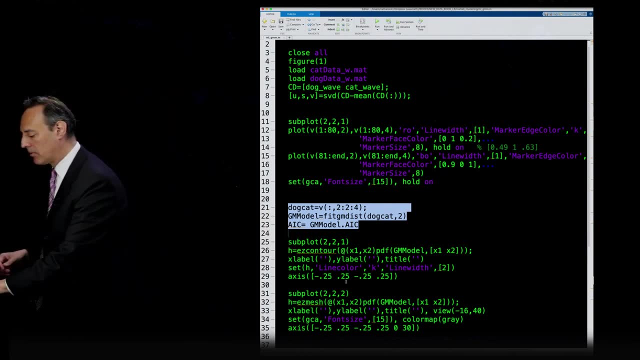 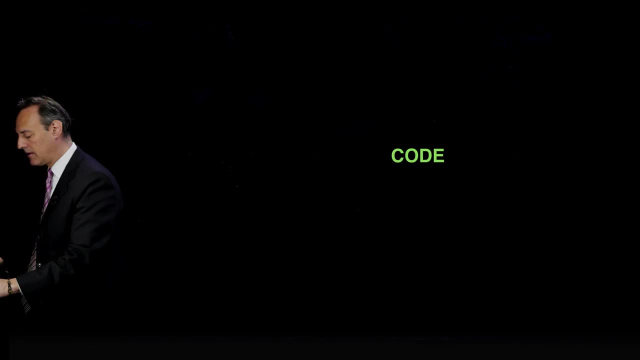 Okay, And so the rest of this is plotting. So I'm going to just show you this, the plots that this generates. actually, they're viewed better in PowerPoint, So I'm going to go look at here. So once she runs that fit, here's the kind of things you get. 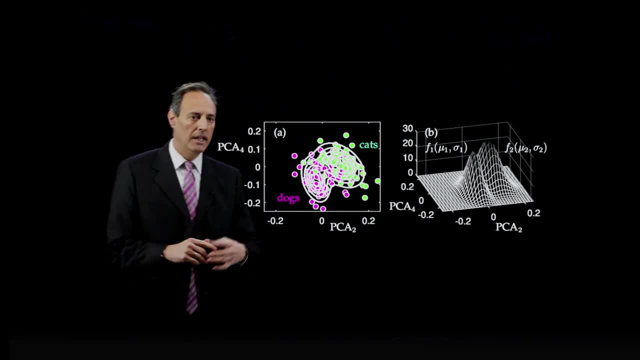 What I'm showing you here is the projection. the magenta and green balls are the projection into PCA space two and four. Remember, those are the two features I extracted out of the Vue matrix and say: let's build a Gaussian mixture model based upon mode two and four projections. 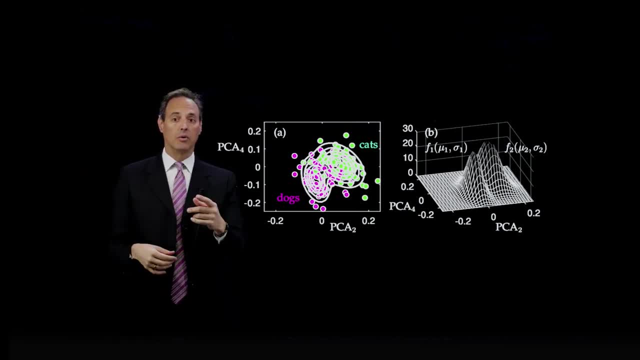 Because when we looked at the histogram of those they had nice separation. So, Again, that was how to set a lecture: five point one, And you can see it here Again: dogs and magenta, cats and green. So what I've done is then I said: okay, take that data fit two Gaussians. 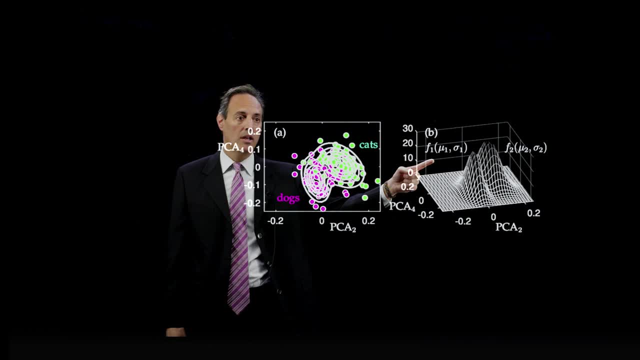 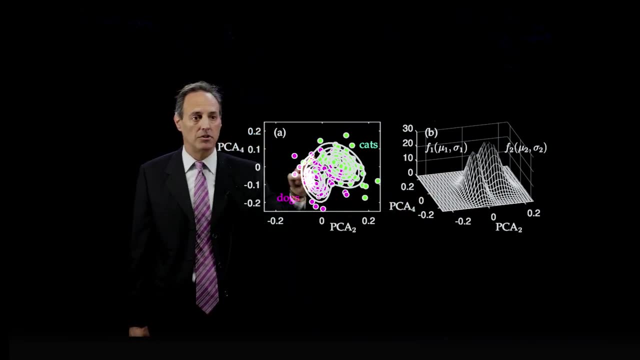 And there they are. So what I have is Gaussian one, which has some mean invariance, Gaussian two, which has another mean invariance, And this, these are the probability distributions associated with this, In fact the contour lines. here are the contour lines of this. 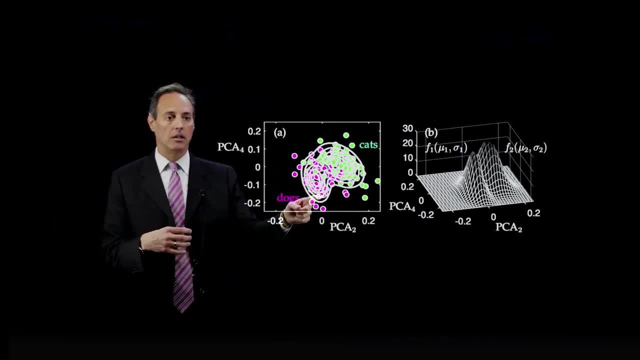 And you can see the Gaussians kept doing a good job And capturing a lot of the behavior you see here. In fact, what you get back is you get mu one, sigma one, mu two, sigma two. So you have those plus the weights alpha one and alpha two. 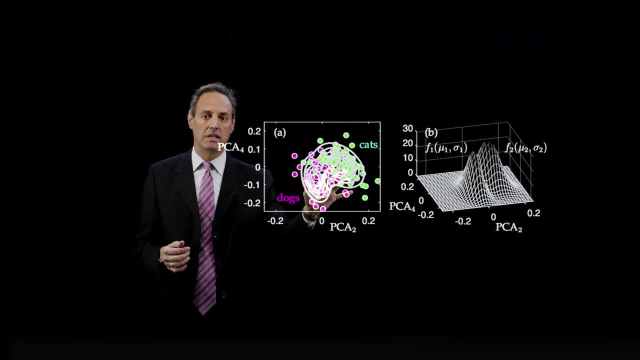 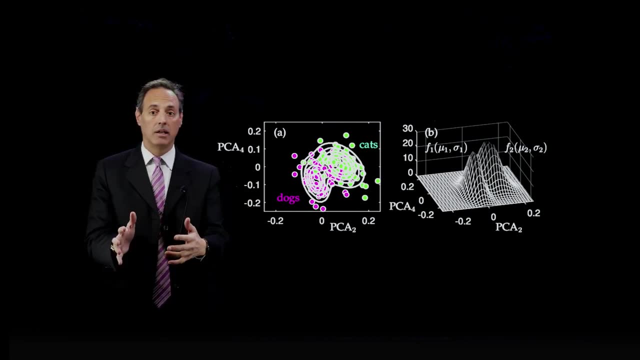 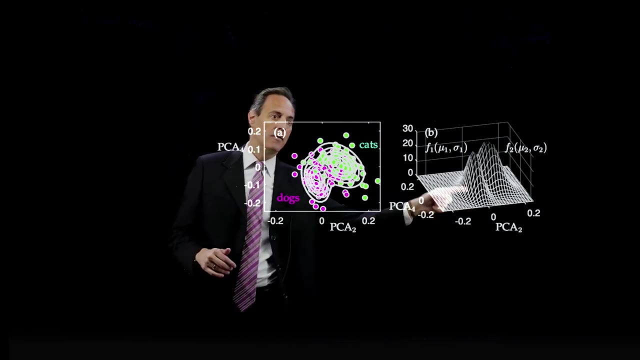 So you get that: six parameters to describe this data in an unsupervised fashion. I did not tell it those were dogs and cats, I simply said: here's these, here's this data set with no labels, And what it tells you is: there is in fact some. 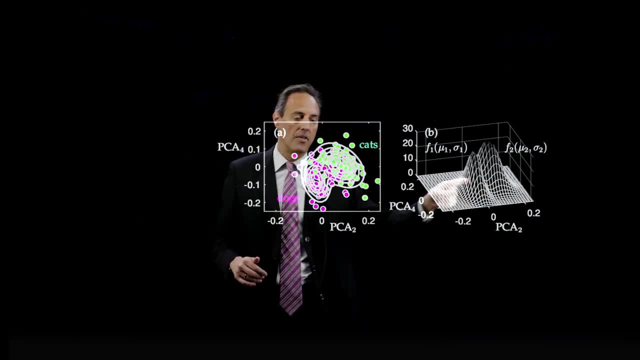 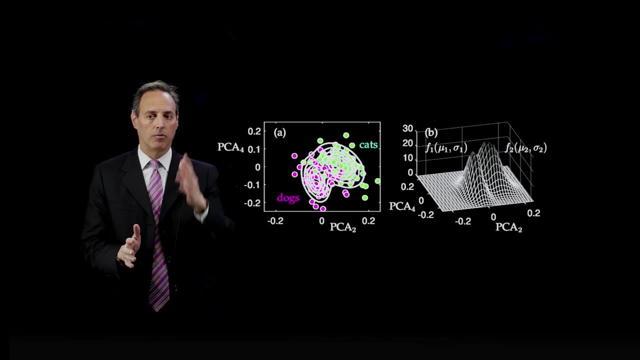 Gaussian distribution of one of the data here plus another one there and runs through here, So again unsupervised. All I gave it was the V2, the second column of V, fourth column of V, without labels. So that's very nice. 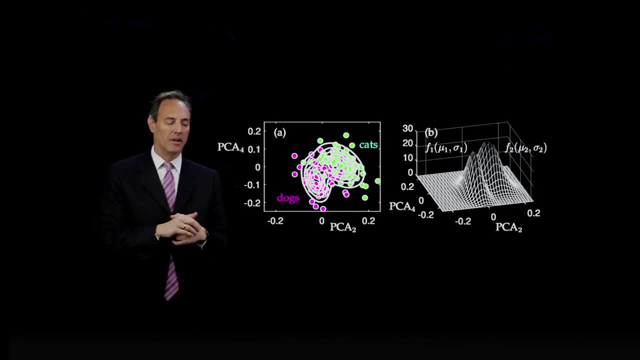 I colored them in because I knew what they were. So that that's the another way to think about it. So what you would see is that maybe I would associate one with the other, and then there's a line of separation between them, right here. 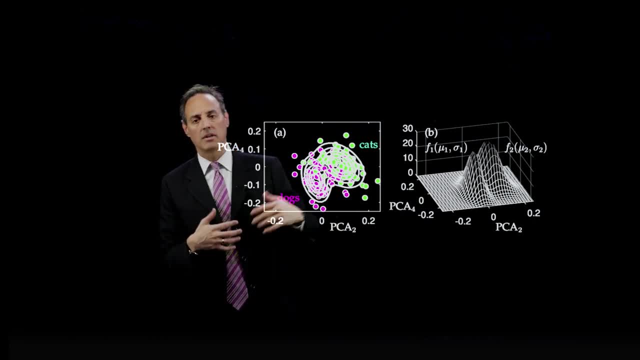 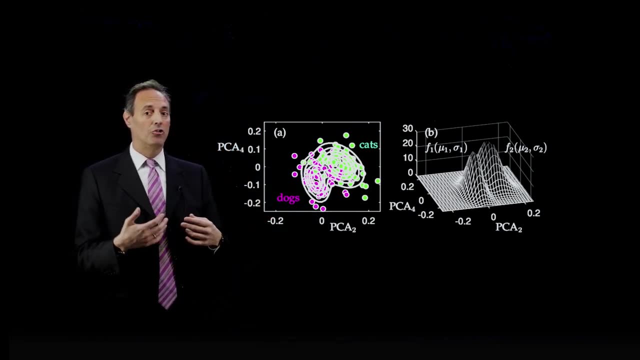 And this is maybe where my decision line would be for classifying one type of data Versus another type of data- But also now, since I have a probability distribution, I could also provide you with uncertainty metrics for this methodology, Which is a very nice thing to be able to do when you make predictions of this sort. 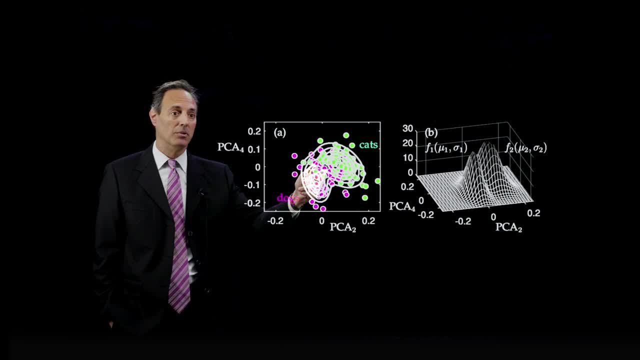 is to be able to say: well, you're down here in this tail of this distribution, the tail of that distribution. How certain am I that it's green versus magenta? And I have high uncertainty when I'm near this line, partly because I know that. 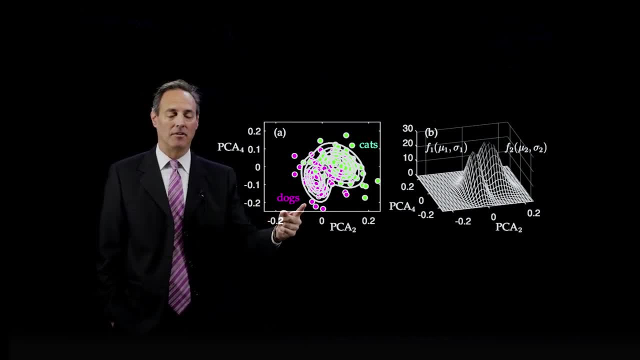 it's going to be either one. in there it could be either one, Whereas I'm going to have very low uncertainty if I'm way out here. I'm pretty certain it's going to be magenta and not green, Because now I have a probability distribution to associate every point with. 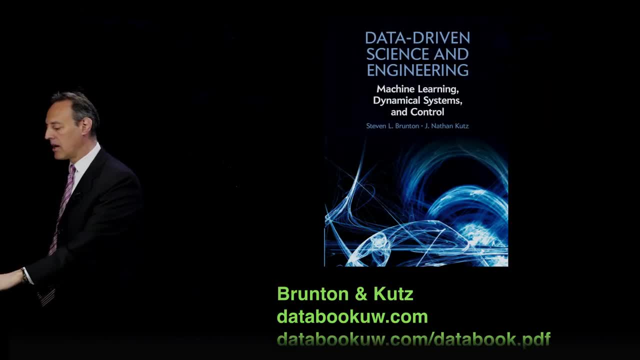 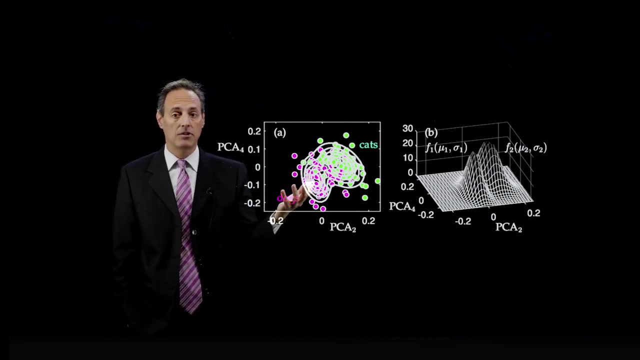 Okay, So that's a nice result out of this Gaussian mixture model. The other thing it also gives you- I said that- is that if you looked, I had it plot out to the screen what the AIC score was. So it not only tells you these distributions, it also gives you. 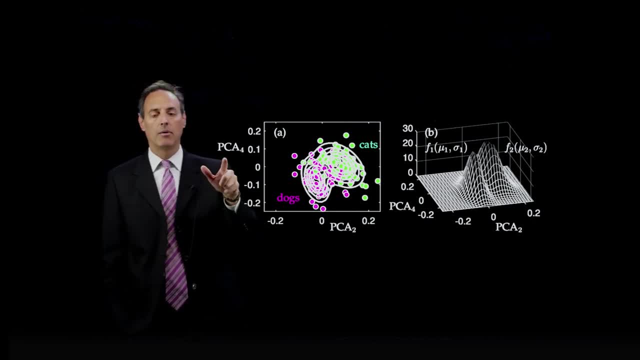 some metric or some information criteria to evaluate that model. So now, if I come back and try different models, you can start saying: well, if I have one model for the data, another model for the data, another model for the data, one thing you might want to do is say which model is the best. 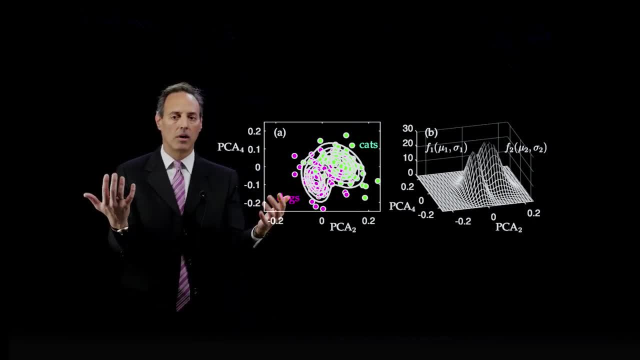 And normally what you do is you compute some kind of AIC, BIC score to evaluate how well they're doing relative to each other, And so that comes out for free out of this GMM mixture stuff. I want to highlight again: this is a really powerful technique.